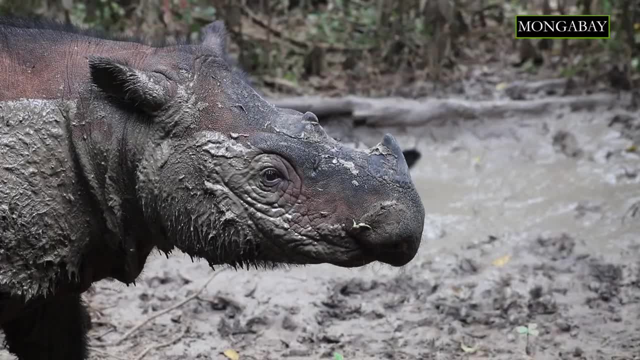 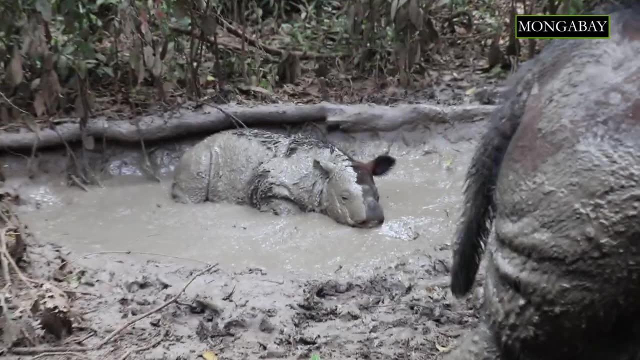 slowing the pace of the population at which the population was growing. But when a population becomes too small and sparse, like in the case of the Sumatran rhino, that can endanger a species too, by making it less successful in reproducing or surviving and slowing down its growth. 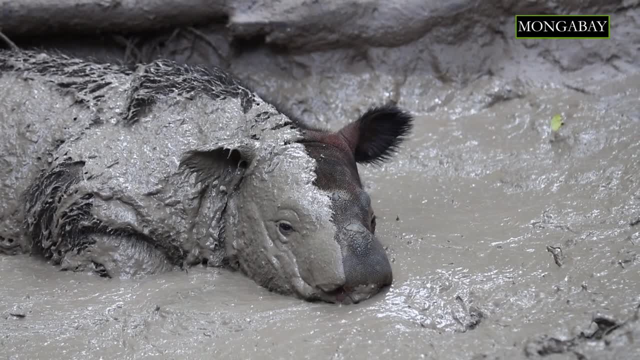 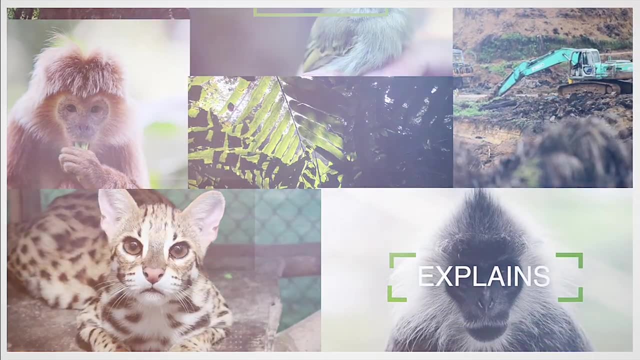 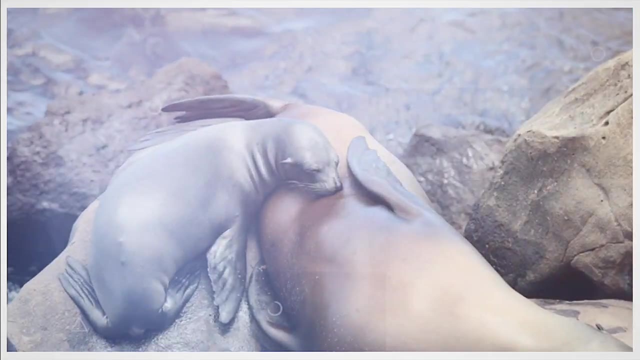 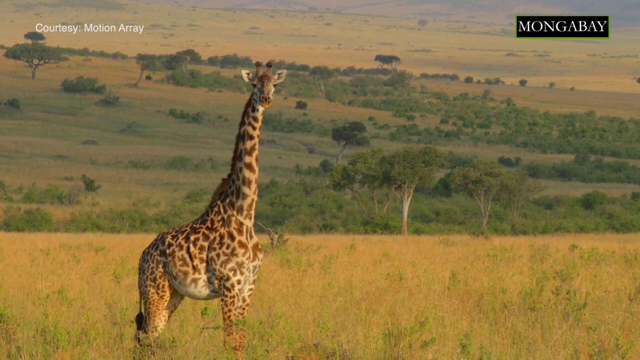 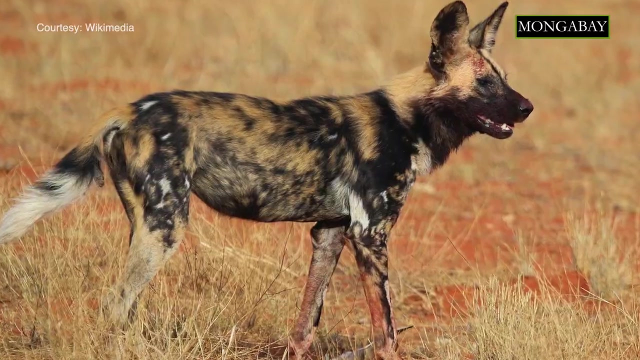 This phenomenon is called the Ali effect and it can trigger extinction. There are several mechanisms behind Ali effects. If populations are small, finding food or defending yourself can become harder, especially if you're a social species Like an African wild dog or a meerkat, Without enough helpers that can cooperate for hunting. 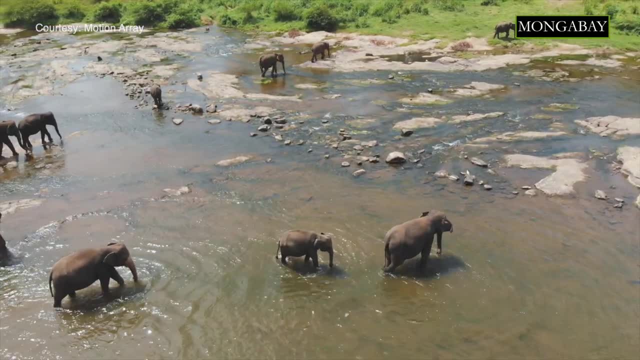 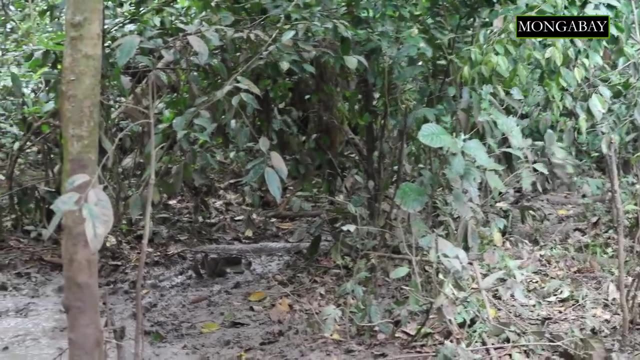 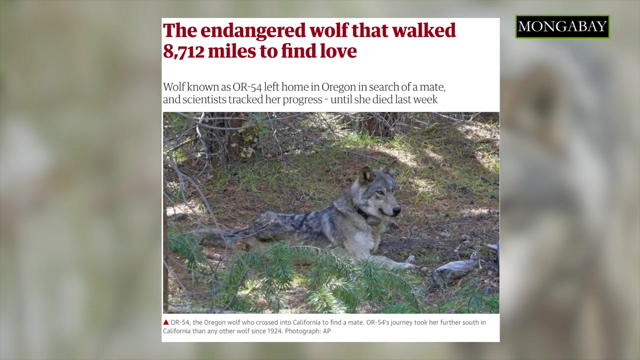 caring for babies, for surveillance or for defending the group against predators. the populations of these species can struggle to survive. It can also become difficult to find a mate when there are fewer individuals in an area. An endangered female grey wolf in the US named OR54 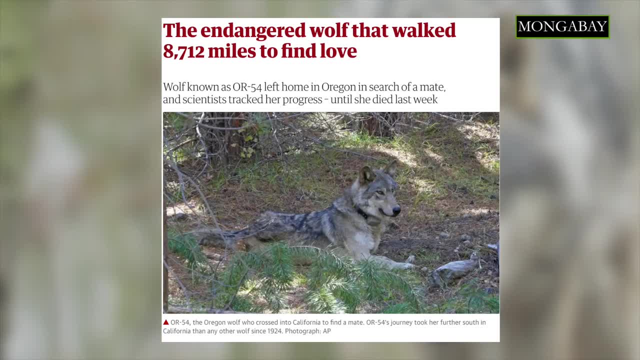 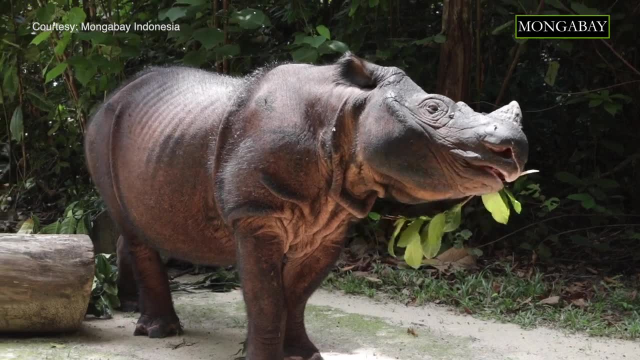 traveled nearly 8,000 miles over two years looking for a mate. She died in February this year and she now lives in a jungle without a partner. Similarly, Sumatran rhinos can have trouble finding mates, since they live in very small. 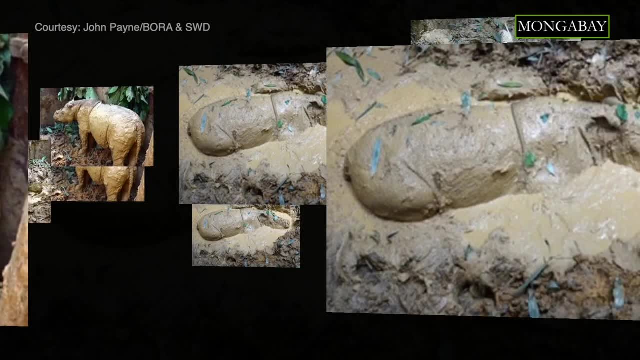 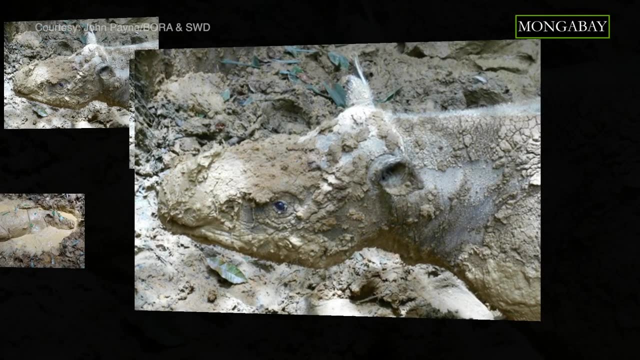 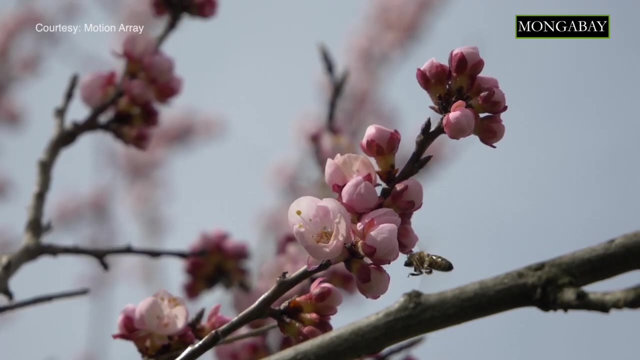 isolated populations in fragmented forests. Iman, for instance, was caught from the wild in 2014 for a captive breeding program, But, as it turned out, she had developed uterine cysts and growths making her infertile, possibly because she'd gone a long time in the wild without mating. 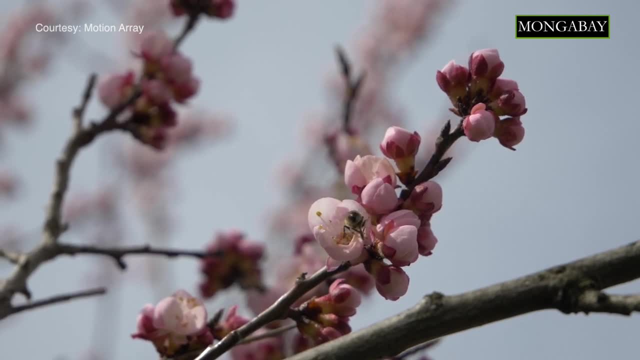 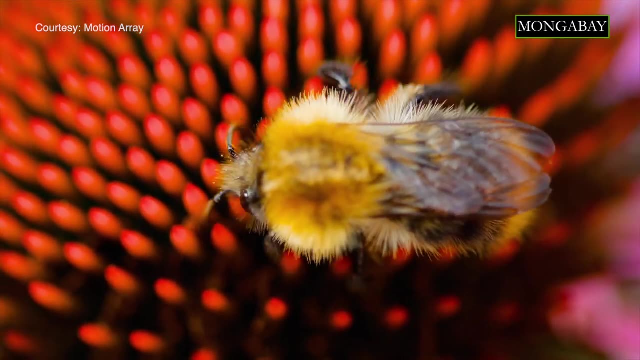 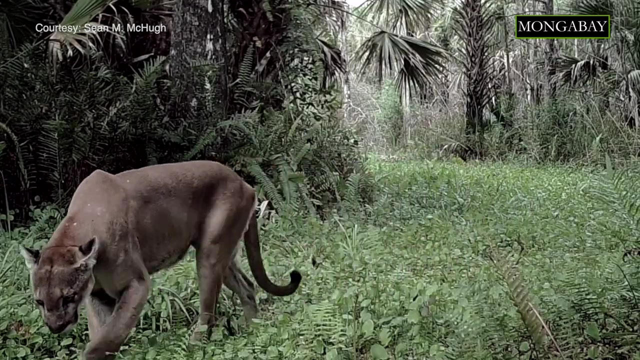 see this effect too. When a plant's population is small and sparsely distributed, the probability that a bee, wind or some other pollinator carries compatible pollen from one individual to another reduces. And it's not just finding a partner that's a challenge. With fewer individuals, 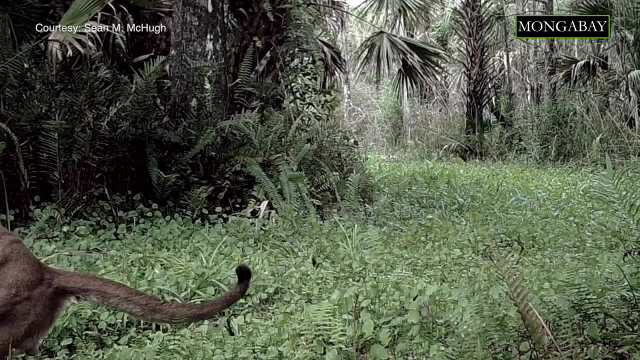 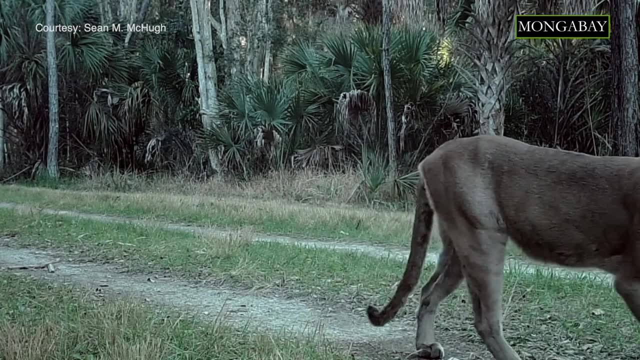 in a population, there's the problem of loss of genetic diversity too. What this means is that as a population gets smaller, the chances that you'll end up breeding with your relative increases. This inbreeding can bring a whole world of genetic problems, And these